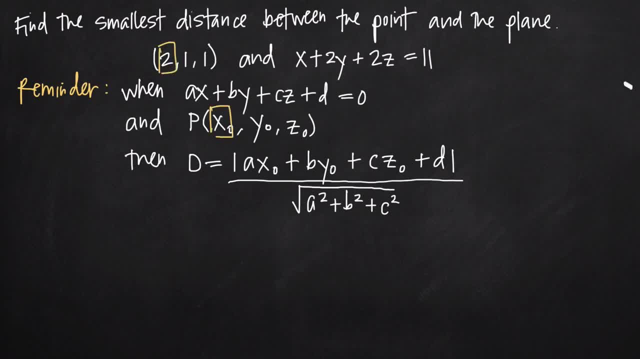 have x sub zero here, we have y sub zero, which is going to be one, and we have z sub zero here. Okay, So we have z sub zero here, which is also going to be one. So those are the three values. 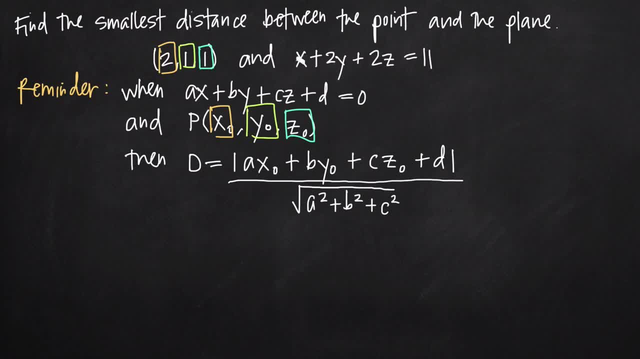 in our coordinate point. Then we can also look here at the coefficients in our coordinate plane equation and what we see is that the coefficient in front of the x variable here is one, so that's going to be equal to a. We have the coefficient in front of y, which 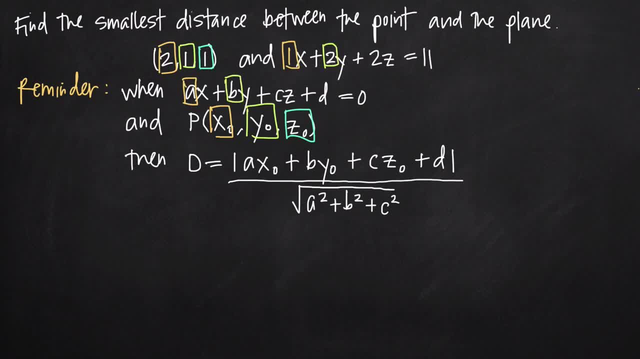 is two, so that's going to be equal to b. And we have the coefficient in front of z equal to two, so c is going to be equal to two. Now notice here that we have plus d, which is supposed to represent our constant. but 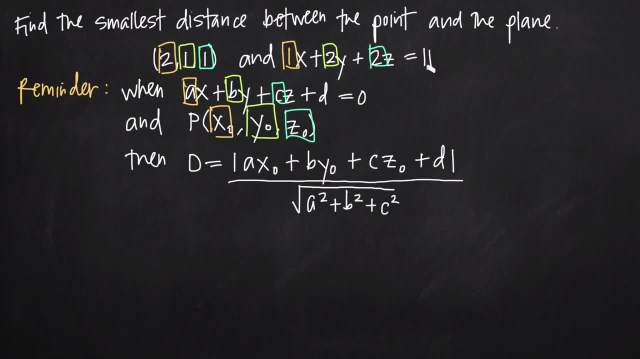 our constant is over here on the right-hand side. So all we need to do is take this constant, subtract 11 from both sides. we get zero over here and we get minus 11 now over on the left-hand side. So notice that the equation of our plane is equal to zero. That's what. 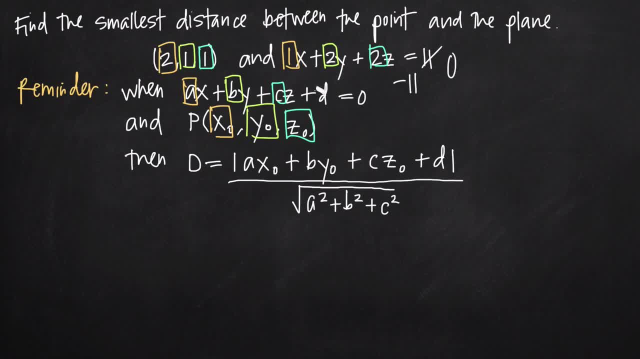 we want on the right-hand side, equal to zero, And now we can say that d is going to be equal to negative 11.. It's really important that we include that negative sign so that we get the correct answer And if you have a negative value in front of any of these coefficients, 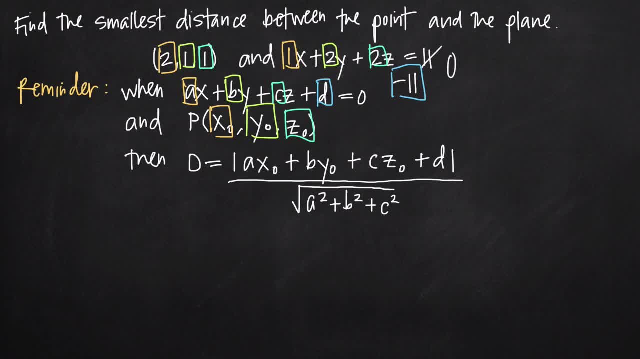 on x, y and z. we're going to want to include that negative value as well. So now that we've identified a, b, c, d and x sub zero, y sub zero and z sub zero, we can plug them into our distance formula. So for d we're going to get: d equals the absolute. 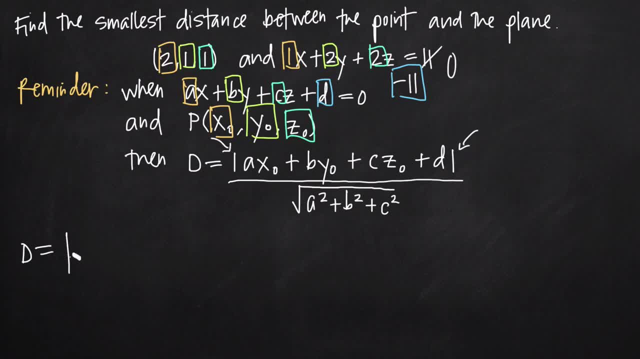 value. Notice. we have these absolute value bars here, So we have the absolute value of a times x sub zero. Well, we know that a is one and we know that x sub zero is two, so we plug those in. Then we get b times y sub zero, So we have b, which is going to be equal. 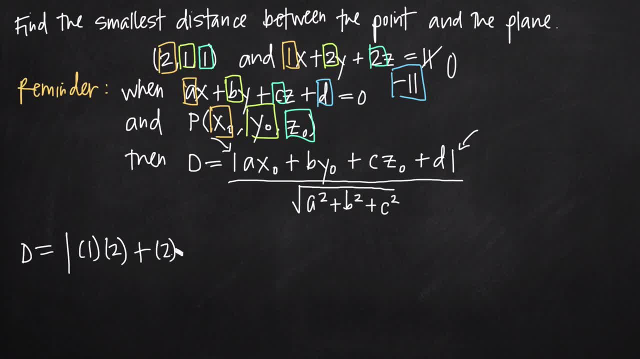 to two, and y sub zero, which is equal to one, so two times one. Then we have plus c times z sub zero. C is equal to two and z sub zero is equal to one. So we get that there. And then we have plus d, So we have plus a negative 11, because we know d is equal to.